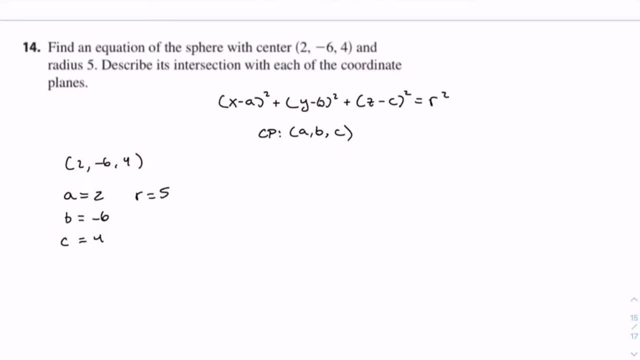 can just literally just plug these right into the formula to get the equation of the sphere, which is x minus 2 squared plus y minus minus 6.. So it's going to be: plus 6 squared plus z minus 4 squared equals r squared r being 5.. So 5 squared 25.. So this is the 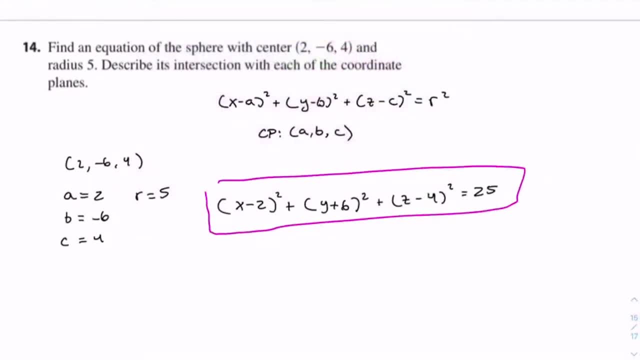 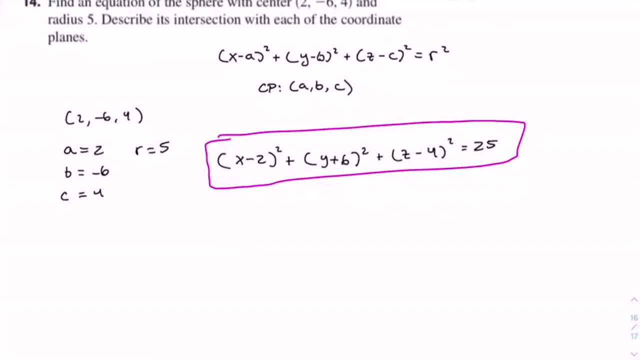 formula of our sphere, So now we need to find what happens when it intersects with each of the coordinates. So we have- let's first start with the xy plane. This means that z equals 0. And all we have to do for the intersection is plug z equals 0, add z into this formula, So we. 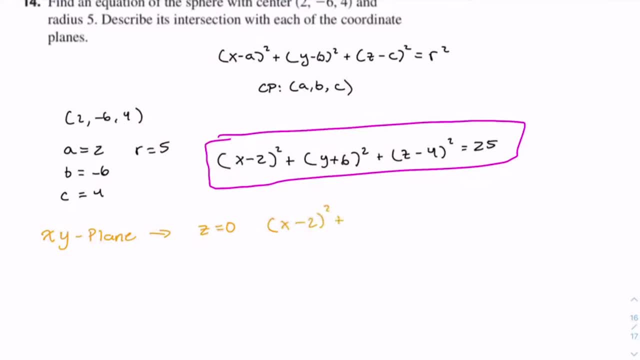 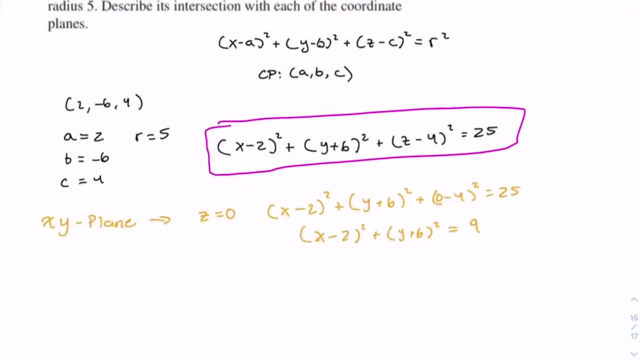 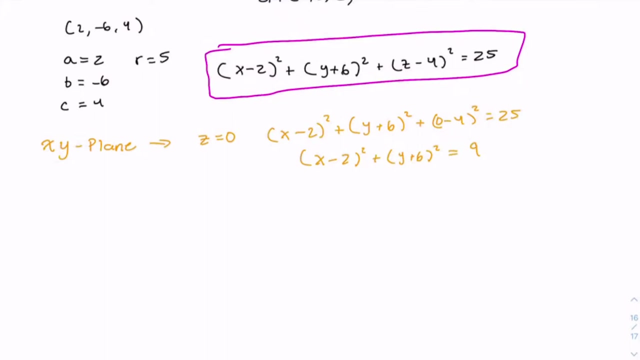 have x minus 2 squared plus y plus 6 squared plus z being 0. So we have x minus 2 squared plus y minus 4 squared equals 25.. And we can simplify this further- equals 9.. So the intersection with the xy plane is a circle, a two-dimensional circle, with radius 9 and 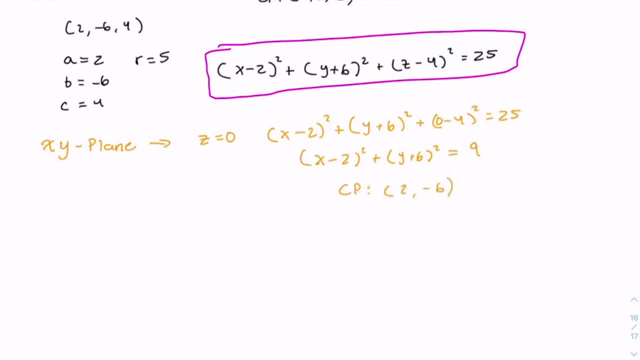 center point being a, b, c. So we have x minus 2 squared plus y minus 4 squared equals 25.. And we can simplify this further- equals 9.. So the intersection with the xy plane is a point 2, negative 6.. Getting that radius's not 9, but a radius of 3.. 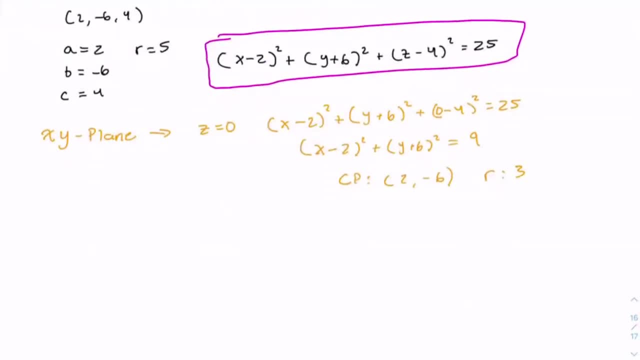 Right. so now let's move on to the xz plane, which means y equals 0, and we can just do the same thing we did previously: plug y equals 0 plus y into the equation. So we have x plus 2 squared plus z squared equals 5 squared x minus 2 squared plus z minus 2 squared plus. 0 plus z squared, which means 2% squared plus z squared. Thus the need to assumed to be equal to die. unitiferrier equals lost. so the number we have to do in our table here is to exercise all the functions of yилась calling. So this is the form of z squared plus. 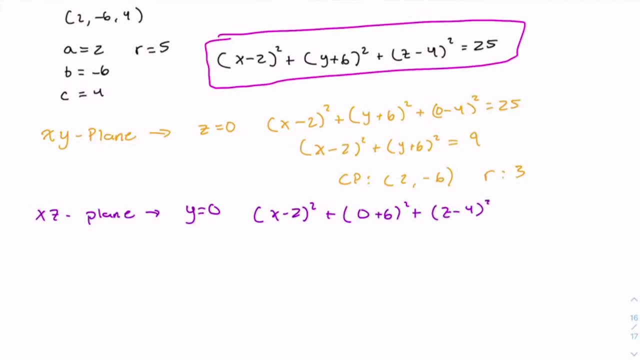 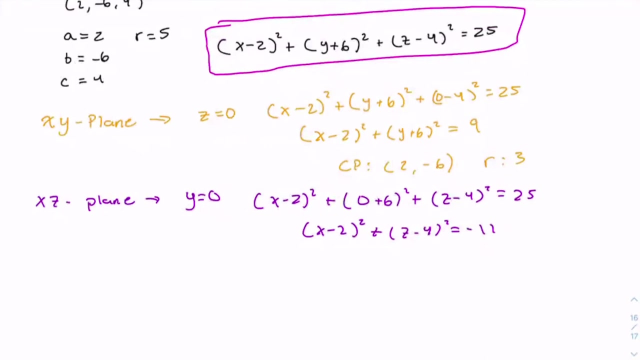 plus z minus 4 squared equals 25.. We can simplify this: x minus 2 squared plus z minus 4 squared equals negative 11.. I don't know if we can have a radius of negative numbers, so I do not think that this exists. 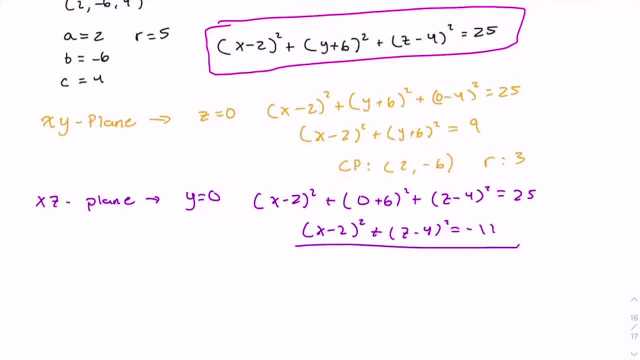 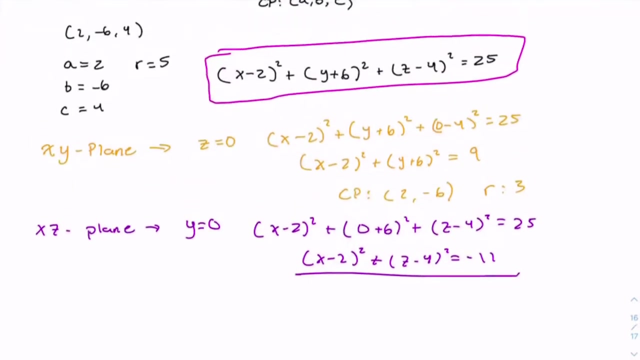 because if your radius is negative, then this intersection must not exist, And we'll take a look at this when we examine it in the 3D graph. So for now we're saying at y equals 0,, this sphere does not intersect this plane. 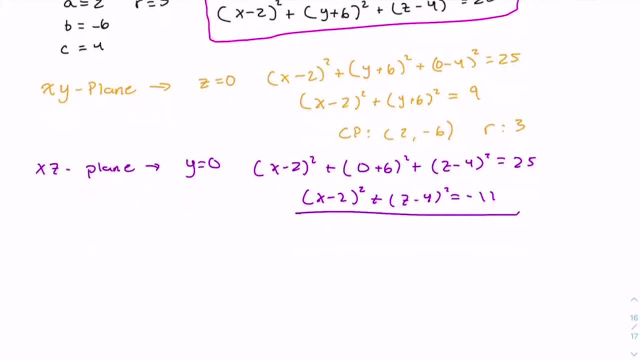 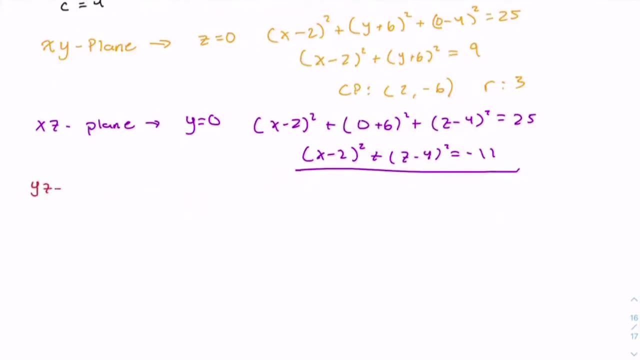 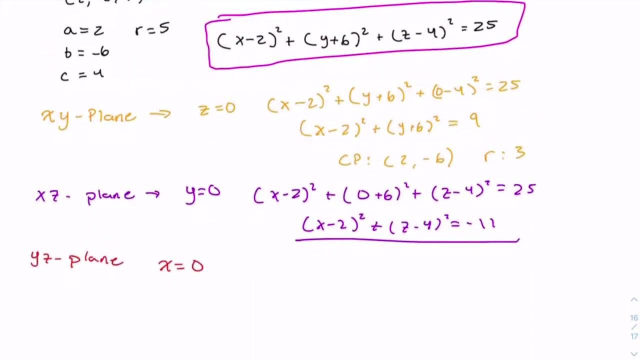 because it doesn't give you a real answer. All right, so let's move on to the intersection of the yz plane, meaning that x equals 0.. And let's plug x equals 0 into the sphere equation. So 0 minus 2 squared. 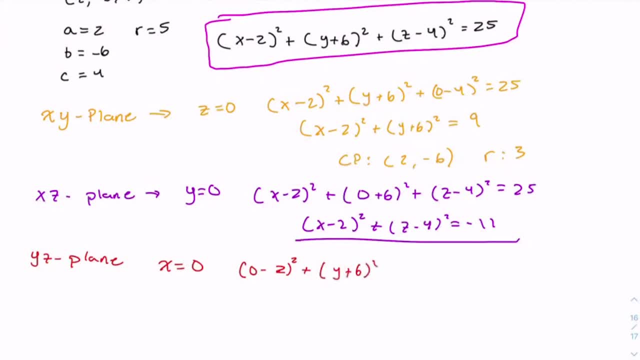 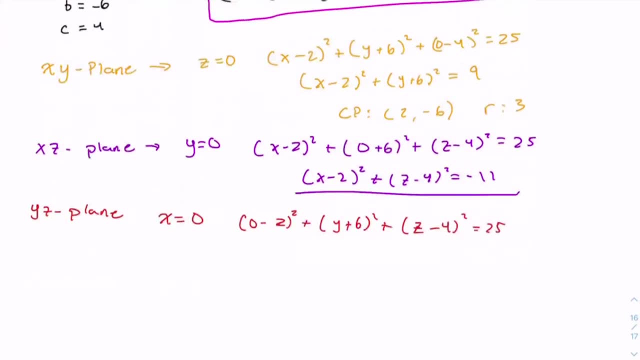 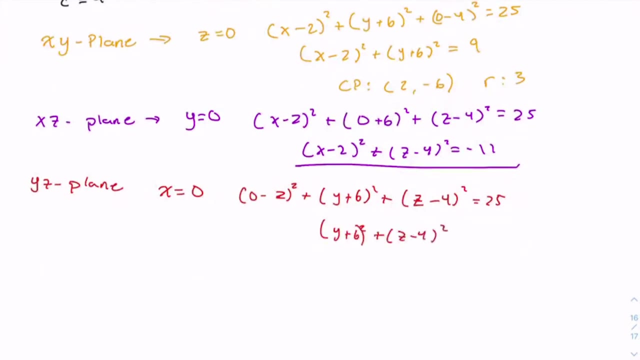 plus y plus 6 squared plus z minus 4 squared equals 25.. Simplify this. We get y plus 6 squared plus z minus 4 squared Equals 21,, radius being square root of 21.. This is a circle. 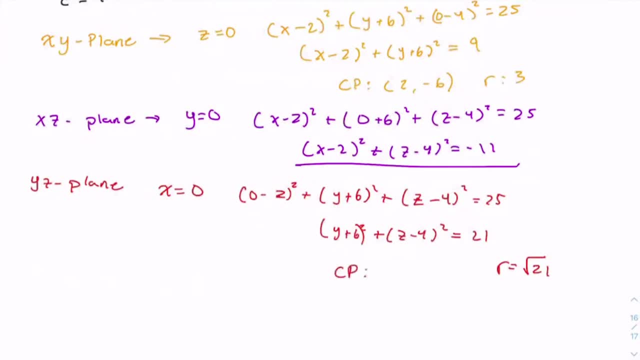 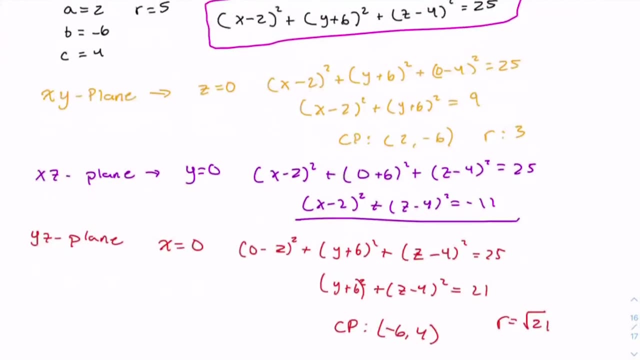 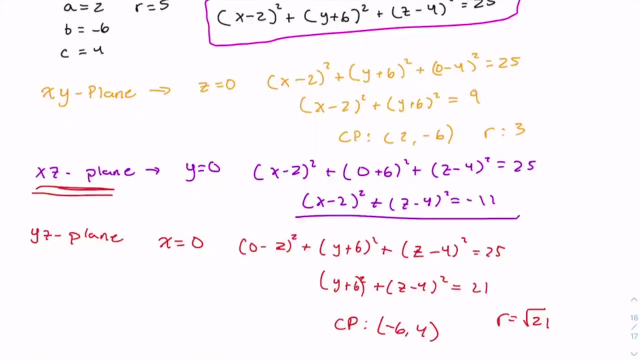 And the yz plane with center point negative 6, 4, with radius 21.. All right, so now let's go investigate this non-real answer right here in a 3D grapher. Here we go, All righty. 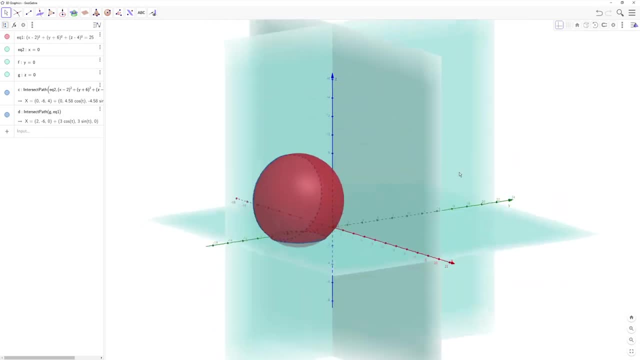 So we have our sphere and we have our intersections. I can already tell that one of these planes does not get intersected, specifically this one, which is the xz plane. So if you have a negative number as the radius, it does not intersect. 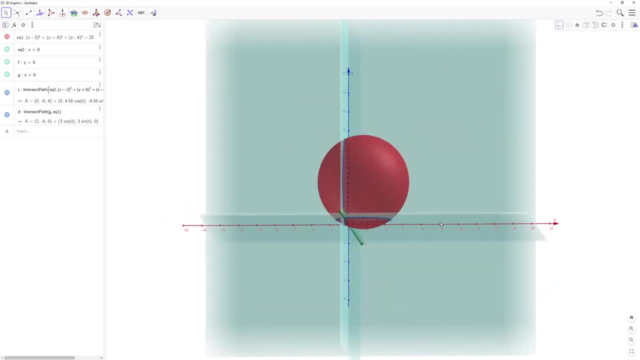 And you can see the other two planes intersect with a circle, just like what we found. All right, Pretty cool.